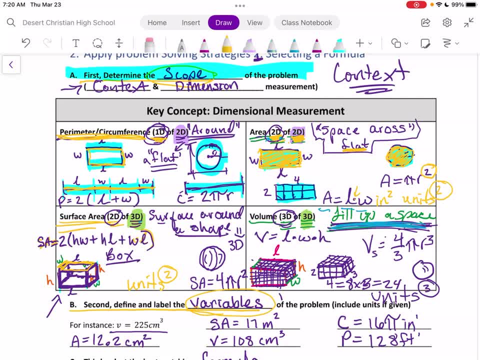 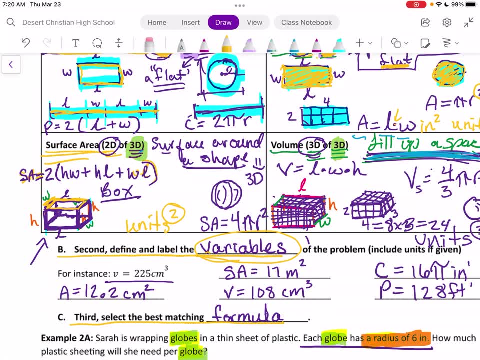 across the table. Okay, so that'd be like a tablecloth. And then we also have the surface area, So this would also be the surface or space, but around a three dimensional shape. So this was like the wrapping paper around all of the surfaces of a box. So we have these three front facing surfaces. 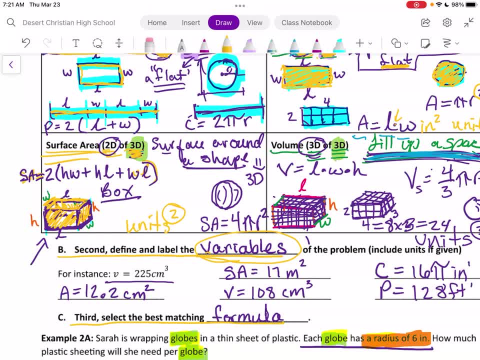 we could see. And then each of these three unique surfaces had its own opposite side, on the back and bottom. So we ended up with this doubled formula here. So each of these were times two, Or we had in the case of our sphere. this is our example. So this would be like: 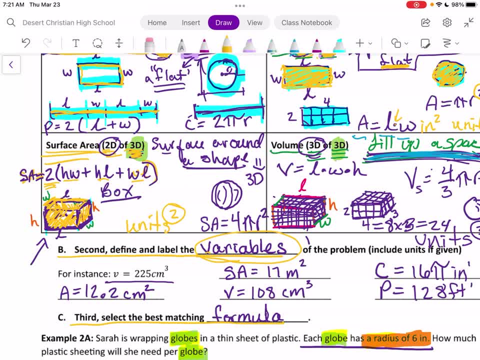 wrapping paper, or example of, like a beach ball. if we filled it up with air, then the beach ball itself, that plastic that is the outer plastic shape around the sphere of the box, And then we would have a sphere of air. And if we popped it and cut it open, that plastic would be the surface. 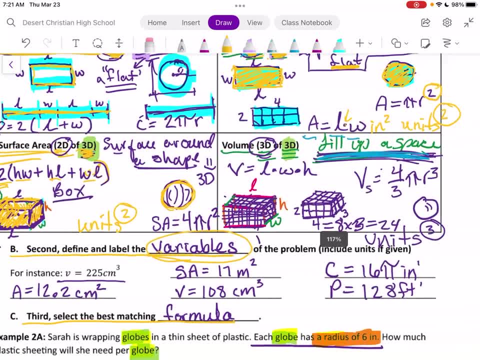 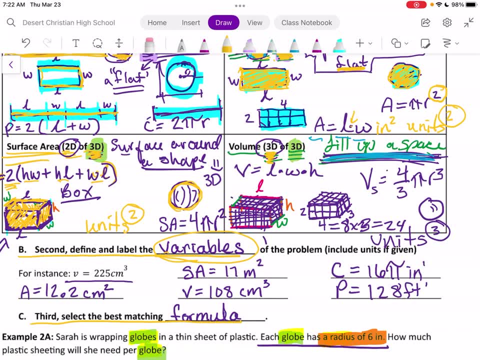 area of the sphere of air. And then, finally, we have volume, that is, the three dimensional, three dimensional measurement of a three dimensional shape. So our rectangular example was of, say, a swimming pool. So if, instead of height, this was depth, 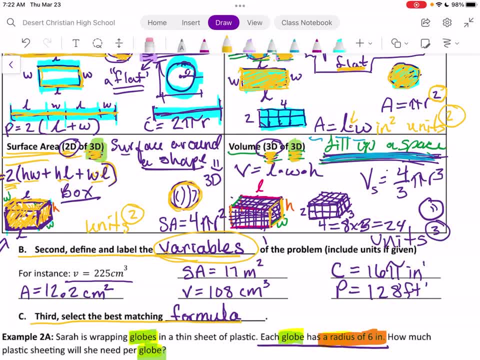 or a height example would be: if you've ever been near the pier, if you've ever gone through the, gone on the coast, been near the cruise terminal or anything, you'll see those shipping crates. Or if you're on the train, if you ever see the train go by, you'll see the shipping crates look like this: 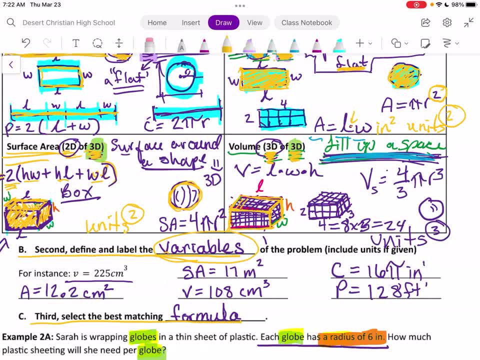 The volume is the amount of stuff that you can fill inside the crate, So that could also be like a moving van or a moving truck, Moving truck. that is the volume, the space, the amount of stuff you can use to fill up a space. Okay, 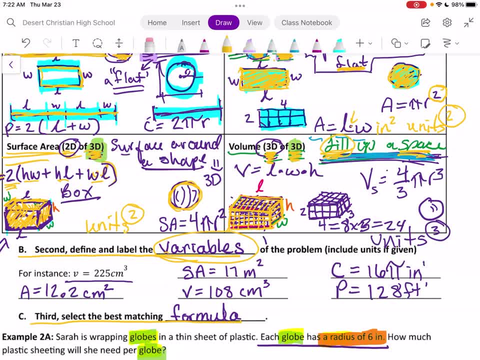 that's the filling of a space In a sphere. that would be like the filling inside a marble, Or if you think of, like a nice round truffle, a chocolate truffle, the filling inside a truffle. I might add that to my Etsy assignment for our next one. 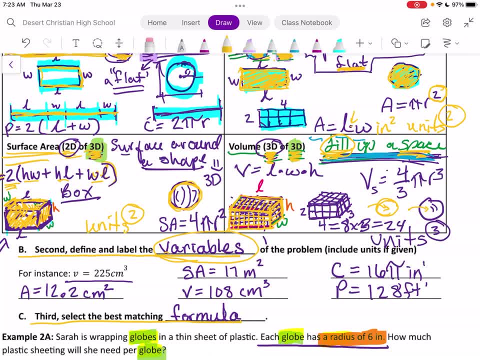 The filling inside a truffle, Anything that's actually filling all the way inside, not just a round, but all the way thick, filling it in. If you're pouring water inside a globe, maybe inside a little like a little fish tank, one of those. 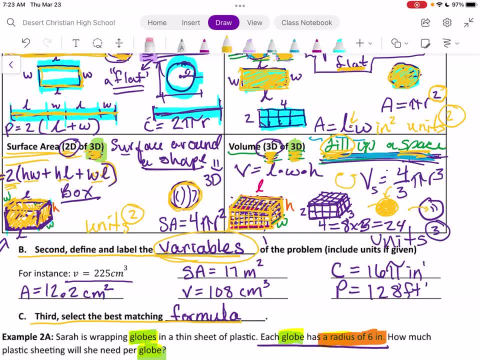 little round fish bowls. okay, that is spherical in shape And we fill that up with water. We're talking about it's filling. that is volume, All right. so that is all about filling. Subtitles by the Amaraorg community. 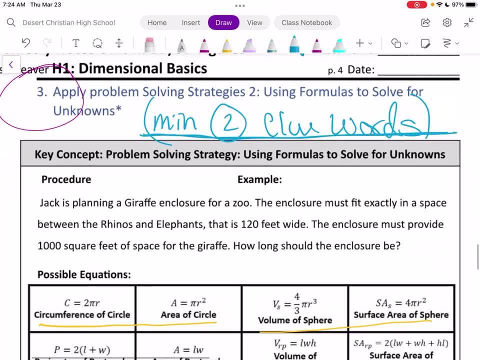 that. yet go ahead and do that before you try this assignment. you can still complete the video, but we're moving on now to applying the solving problem, solving strategies and for these purposes- because I'm not here- we're only going to do the first half of this, which is just the formula, so we're just going. 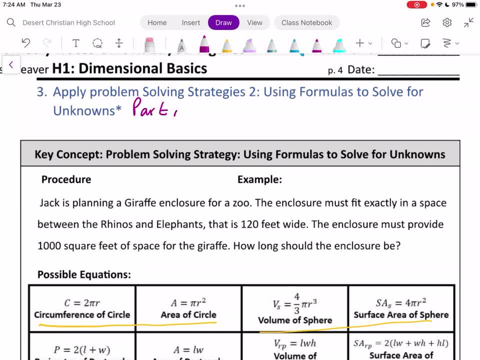 to call this part a. okay, part a, we're going to keep it the simple part, which is just the: the formula set up, the formula set up. the part B. that we're not going to do today. we're going to save this for when I'm back. which word? 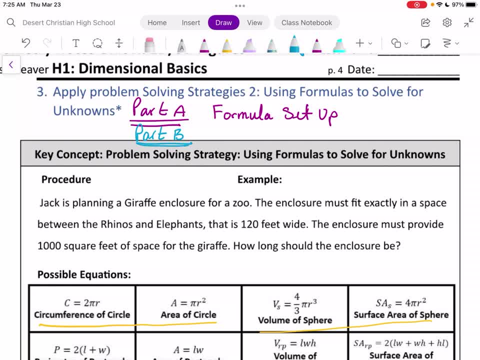 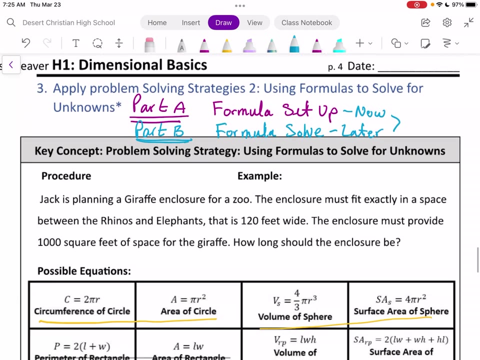 willing should be Monday, it's looking good. part B is the formulas solve, and this is going to involve music, music, music, music, some algebra, and this will be later. okay, this is gonna be now, all right now, and later together they make a candy that literally pulled one of my teeth out. 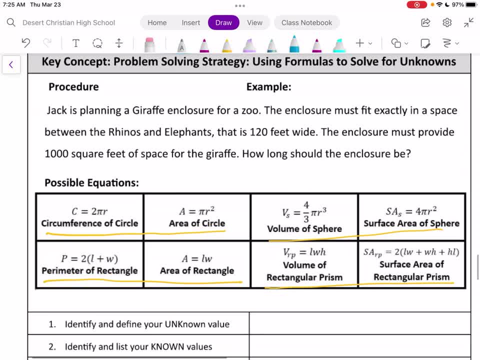 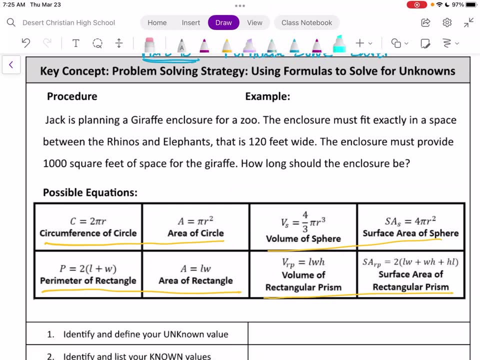 once. so nice little bit of mrs weaver trivia. so let's go ahead and take a look at this. here is our problem-solving strategy: using equations, using formulas to solve for unknowns. okay, now we're going to have and we're gonna, I'm gonna. 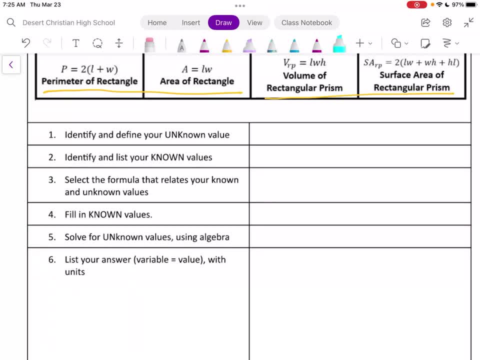 jump down and kind of look at our formula, our procedure up front and then we'll look at the example. so our procedure here: we want to start by identifying- and I did defining- our unknown value. basically, we're going to ask ourselves: we're gonna look for what is the question mark of this question? what are they asking us to? 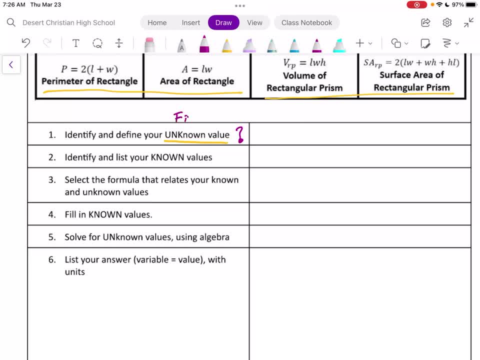 find. what are we finding? we always want to start with the end in mind. what is our goal? all right, and if you are maybe taking this in a future course, you might want to start with the end in mind. what is our goal? all right, and if you are maybe taking this in a future, 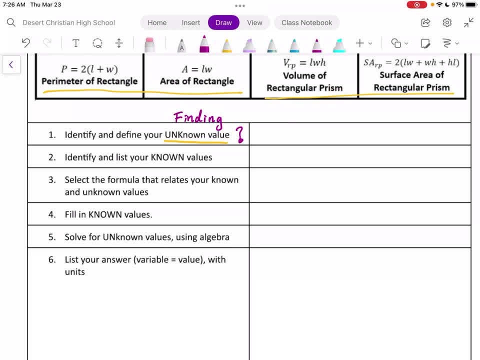 class are really have emphasizes with my algebra class this year with word problems. we always want to start with defining our unknown value. then we're gonna look and find: well, what then? what are our known values? and we want to identify a list. when we say identify, unless that means with a variable. so 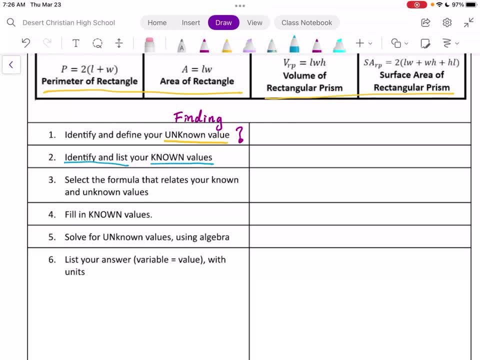 we're going to find our known values, we're going to list those of variables and then we're gonna select the formula. so this is where we're gonna go back to that H two process, where we need to look at our context or the scope, whichever you want to think of that. 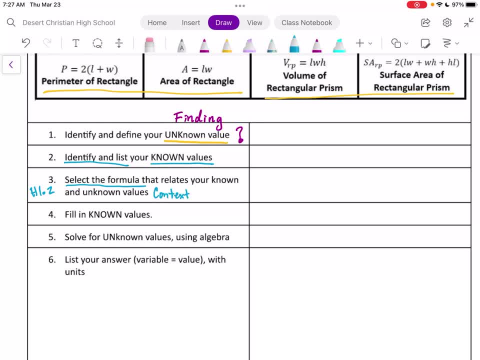 as the context, okay, and the dimensions of the problem. Is this circular or rectangular? Do we have a 1D, 2D or 3D measurement? Is our object two-dimensional or three-dimensional? And use that to select the right formula. and we're going to double-check that by checking our 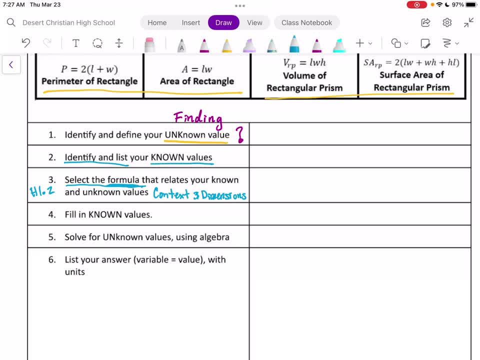 unknown value and our known values and make sure all of those match up with our formula. And then this is the big key, right here Please put a star. here We're going to fill in our known values. So this is going to connect back to those important points from our very first two units. 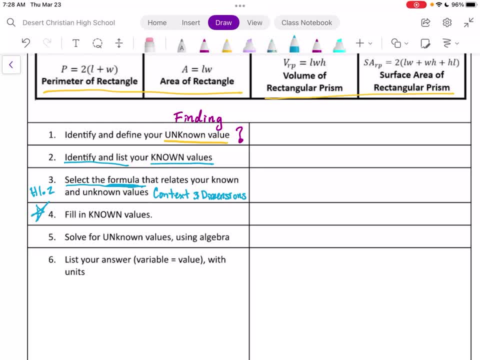 where we say: we don't just plug numbers anywhere And evaluate an expression. We are filling in our known values, and I want us to add this here in the equation: This formula is an equation, All formulas are equations, And by that I want to. 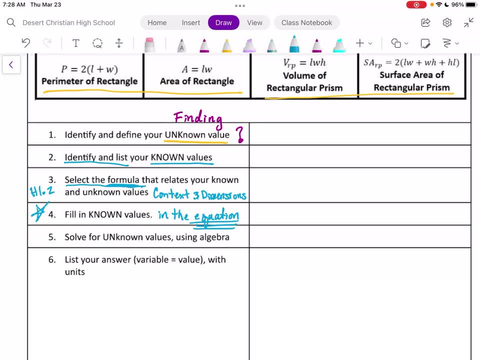 emphasize: we have two sides of an equal sign. Don't just ignore one of the sides. That is the number one mistake that students make, and I created this equation to make sure that we have an equal sign. This lesson here is not directly from the textbook, because the textbook assumes 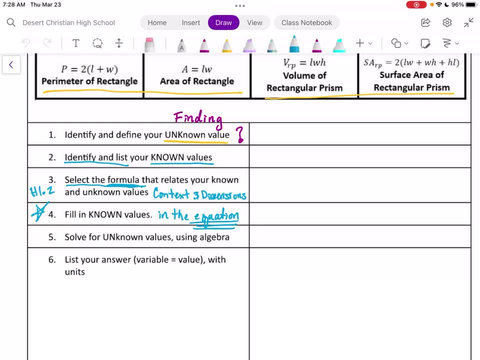 students are going to do this, And I found that so many students didn't, and then they struggled with everything else. So I created this lesson to make sure that we don't take this for granted, that we actually practice this step, that we do this step, These two steps here. 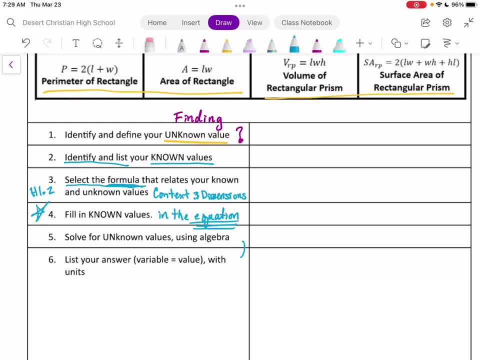 first of all, these box sizes should be swapped, so we'll deal with that. But these two boxes are going to be done later. This is part of our later in the now and later. okay, So we'll do these later. We're just going to focus on one through four. This is what your exercise is going to be. 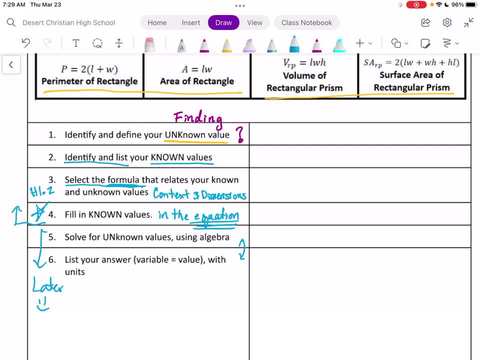 on today. all right. So with that, now that we understand we're looking for our unknown value, We're going to label our known values, We're going to select a formula that matches, and then we're going to fill those in. Once we've completed number four, we should have an equation with one. 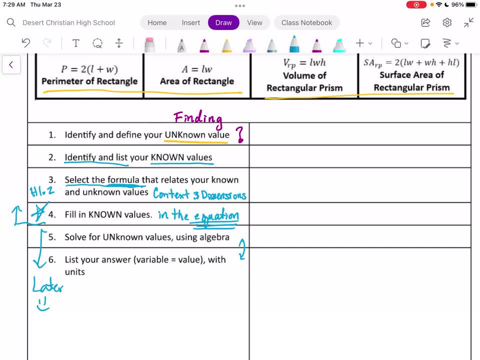 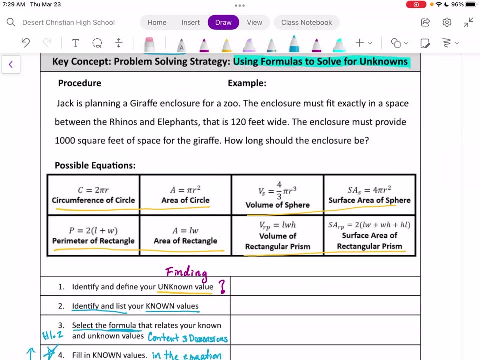 known value and every other value known, so that we can then solve for our one unknown value. That is our goal, okay, So let's take a look at this example. We have an example. Jack is planning a giraffe enclosure. No lions guys, all right. So Jack is planning a giraffe enclosure for a zoo. 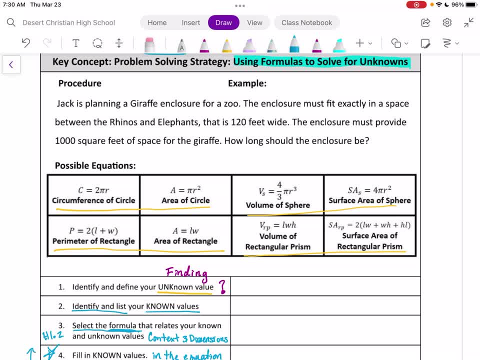 And we'll see that this comes from our previous example. The enclosure must fit exactly in a space. sorry, that's the alarm I have going there. The enclosure must fit exactly in a space between the rhinos and elephants that is 120 feet wide, The enclosure. 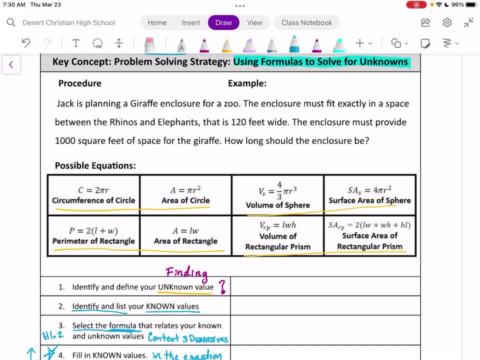 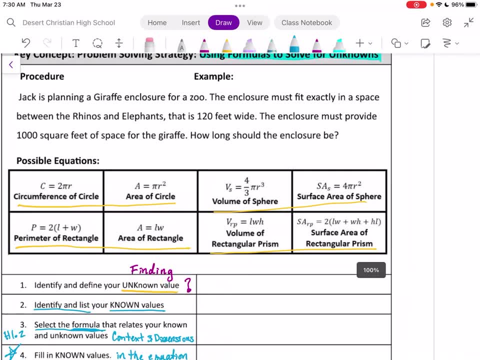 must provide 1,000 square feet of space for the giraffe. How long should the enclosure be? And I always find it helpful. I'm going to kind of go off of my margin here to think about how long should the enclosure be, And I always find it helpful. 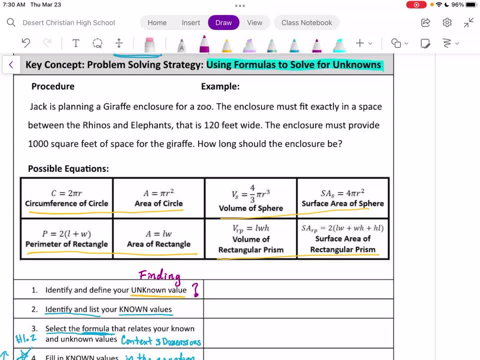 I'm going to draw a picture for these kinds of questions. So I have, and we did this in the previous video, but I have some space between rhinos and elephants. I said before it makes sense, based on this information, since this space is 120 feet wide. okay, that if they say it's 120. 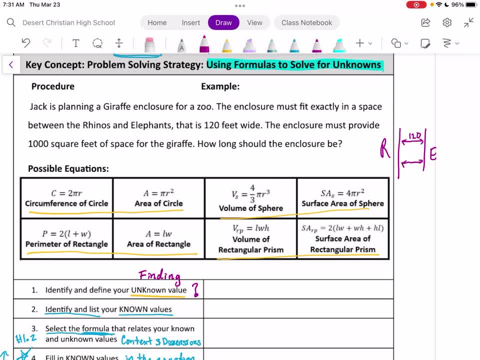 feet wide. that would imply it's consistent. So I'm going to draw a picture for these kinds of reasons. If they're saying it's consistently 120 feet wide, oops 120.. There we go, which would imply that this is a consistent kind of that. these lines are parallel, equal distance apart. 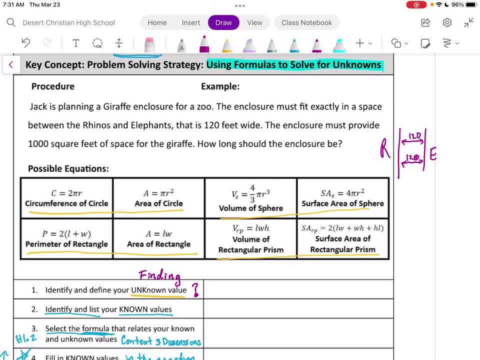 okay. So this gives me a little bit of an idea of sort of shape. So this gives us just enough to kind of get started. And let's start with step number 1.. And I'm going to go with since I let's look at our clues in yellow, identify and define your unknown value. 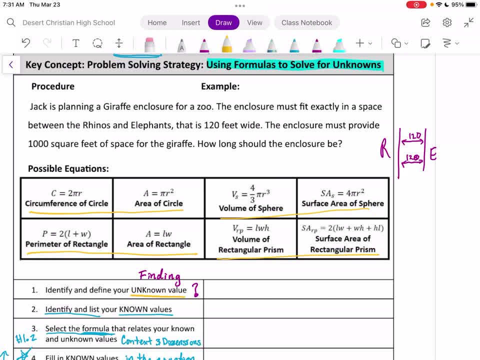 and our clue here is the question mark. so where is my question mark in this question? my question mark is here, so let's look at this: how long should the enclosure be? what variable of all my possible variables here: circumference, radius area- I've raised again volume radius again. surface area: raise again. 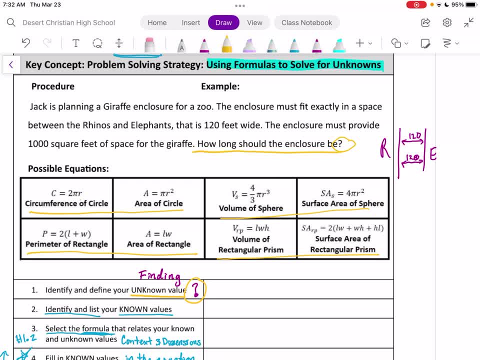 perimeter: length, width, area length: width- again volume length, width, height, surface area- again length, width, width, height, height, length. alright, so we get an idea of our different types of variables. which of these variables would be included here? and I should see that long is idea of length. so my unknown variable that they're asking me to find is length. 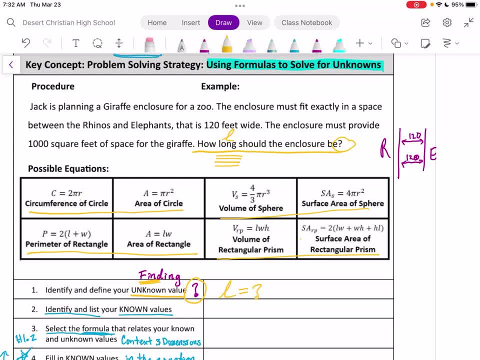 so length is my unknown variable, and that's what I want to start figuring out. is: what is it? what's my unknown that they're asking me to find? okay, so that's done. great number two: identify and list my known values. so now I'm going to go back through my example, my problem. 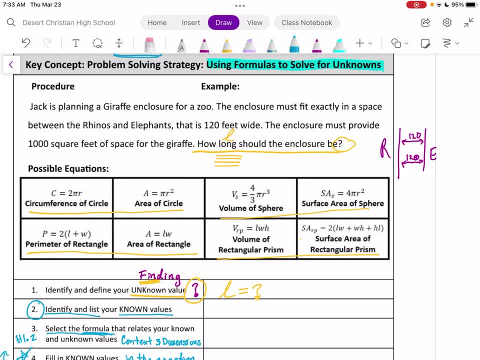 I'm going to look for any other values that they give me, and values are usually going to include numbers. we'll look at some more complicated examples later together. for this one, for our first few, for your problem, they're going to be numbers. all right, so let's look at other. 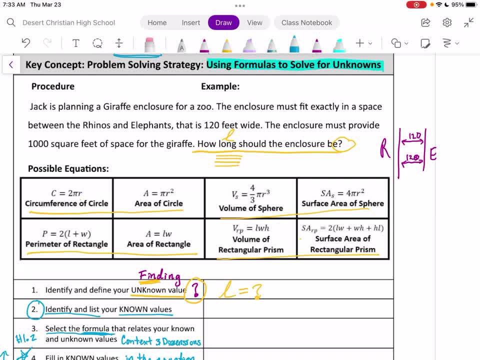 numbers in the question and I'm just going to start by underlining phrases that have numbers. so I have that is 120 feet wide and must provide 1,000 square feet of space. okay, so if I look at 120 feet wide, which variable would 120 feet? 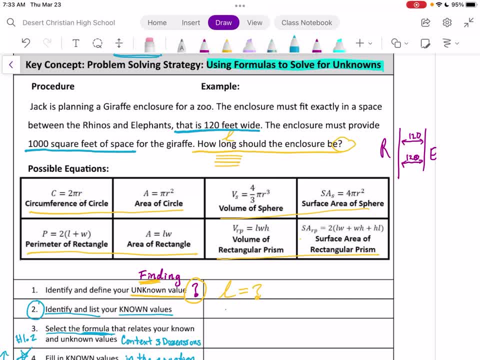 wide, so I can kind of put: okay, something equals 120 feet. which variable would that be? I mean, maybe let's list our possible variables, that might help us. we have circumference as a variable. radius, area: radius again, volume, radius again. notice that PI is not a variable, it is always the same. 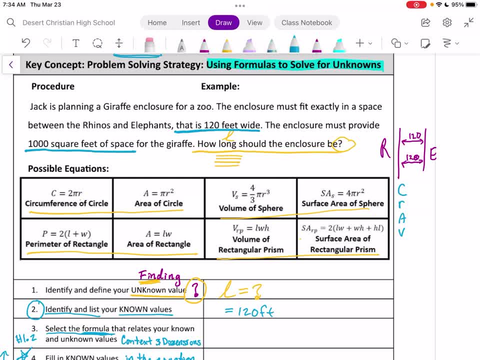 value is three point one, four, one, five, nine, six. it's not a variable, it is a symbol that represents a constant value: radius again, surface area radius again, perimeter length, width area again. volume again, height, surface area again. so these are all of the possible variables for these, this initial assignment h1. okay, is all we're going to. 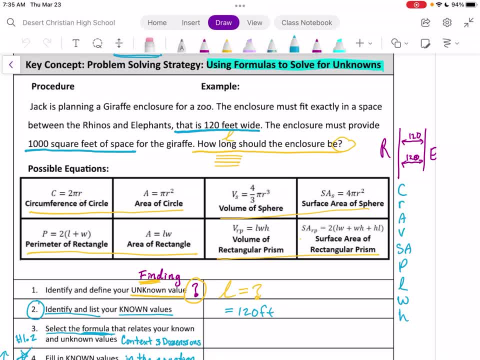 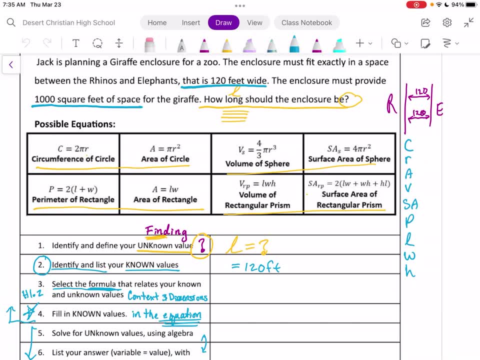 have in h1, which is the initial value of h1, and h1 is the initial value of h1, so h1, our initial value, is the set of variables, so we're keeping it limited. which of these variables would 120 feet wide most likely be referring to? and 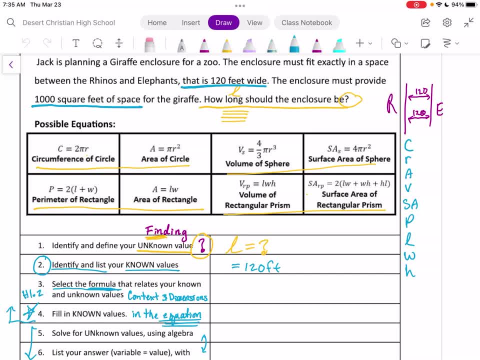 that would seem to be width. okay, wide would be with. so we'll say width is 120 feet. then we also had 1,000 square feet of space. okay, now this one can be a little bit trickier. space, well, space. we want to think back to our context. space. 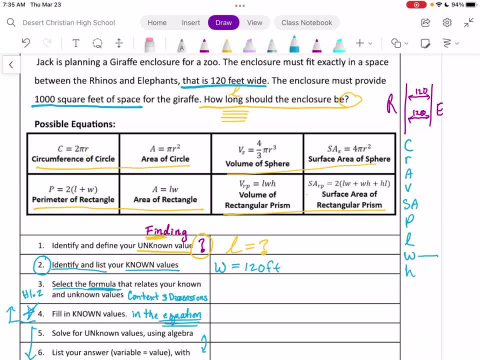 could be some. it's going to be some kind of an area thing, so that could be area or surface area. so we might want to pause here and actually look forward to our context. let's think about the situation. so we're going to put here that we have something as 1,000 feet squared. we might 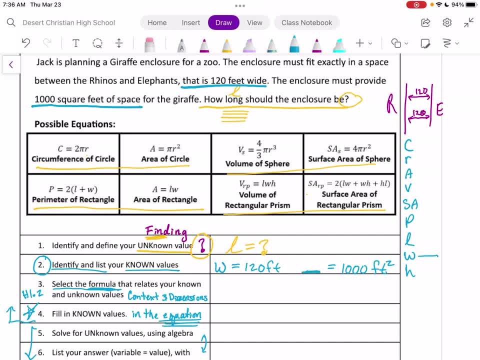 not be exactly sure whether this is area or surface area. we can come back and maybe figure that out in a moment. so let's look into our formula and understand our context and dimensions. okay, so looking back, remembering for context and dimensions, we had a few steps that we had to take to understand our context and dimensions. so let's look back. 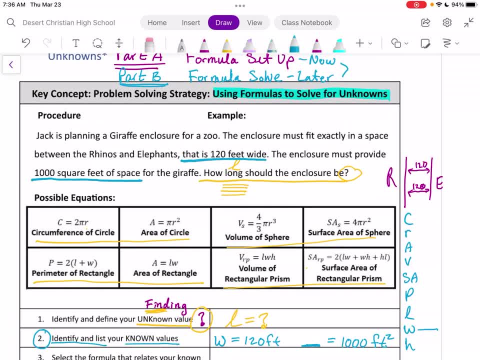 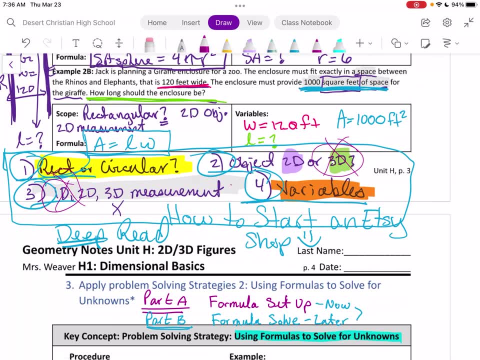 and look at our formula and understand our context and dimensions. okay, so, looking back for this- and I'm gonna recap them kind of up in the corner here- we wanted to check, and let's look back up here real quick: is a rectangular or circular? is the object 2d or 3d? are we dealing? 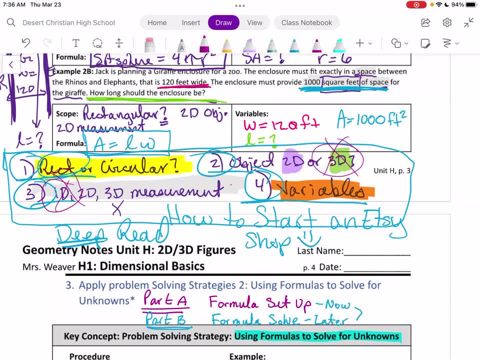 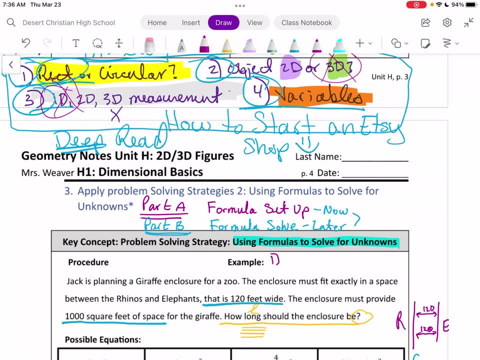 with a 1d, 2d or 3d measurement. and then what are our variables, which we've started that process, so I'm gonna kind of cat recap those here. is it rectangular or circular? is it is the object or one? sorry, 2d or 3d? is the measurement 1d, 2d or 3d? and then number four was the 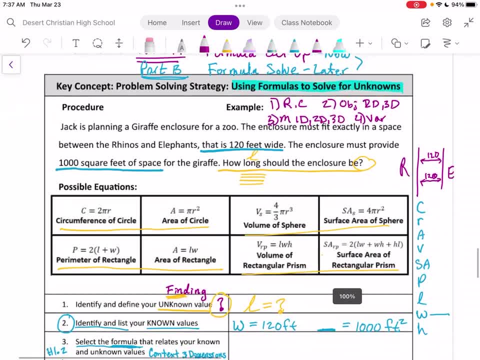 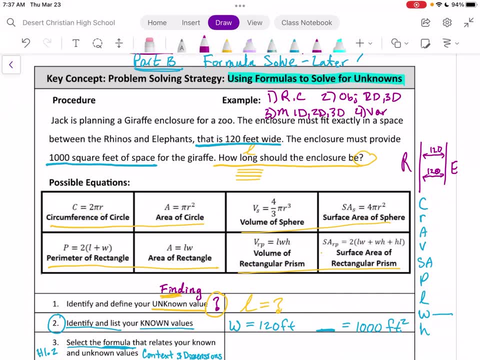 variables. okay, so is this situation rectangular or circular? well, looking at our giraffe enclosure, since we're dealing with a space between parallel lines and we're being asked how, if this is the width, and we're being asked how long the enclosure should be like, if this is my, see how important drawing that picture is, if this is my. 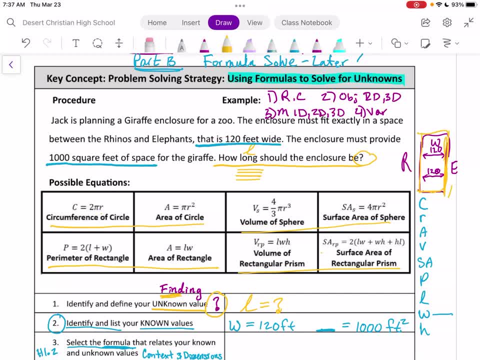 question mark length. okay, well, this forms a rectangle, so this looks like a rectangular situation, which means the circle formulas are all out, all right, so we've just eliminated half of our options. that's helpful. okay, then, is our object two-dimensional or three-dimensional? so this giraffe enclosure- and we discussed this in the previous video- there's 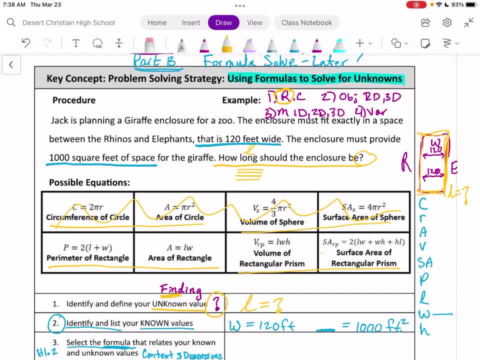 nothing here about there being a roof to the enclosure. there's no mention of a height to the enclosure. um, um, um, it's not a cage. there's no depth, we just have a width and a length. there's nothing that indicates a third dimension to the object, so everything would seem to. 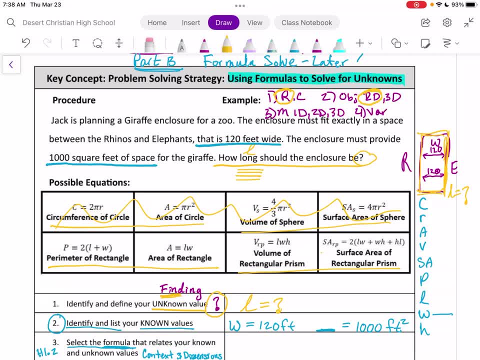 apply. this is a two-dimensional object, so two-dimensional objects are circles and rectangles. three-dimensional objects are spheres and prisms. so this would seem to eliminate prisms and spheres. so now we're down to perimeter or area of a rectangle. then our next one is: are? 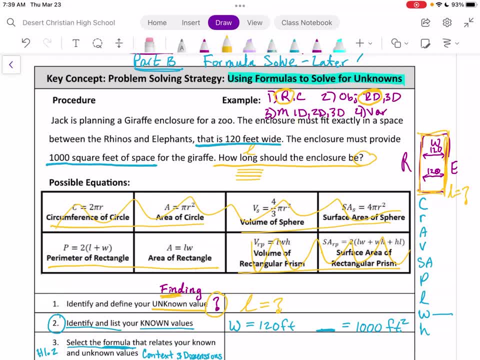 we measuring: a one-dimensional measurement, a two-dimensional measurement or three-dimensional measurement? remember I said we cannot have more. we can't measure more dimensions of an object than an object has. so if we are have a two-dimensional object, we cannot take a three-dimensional measurement. so 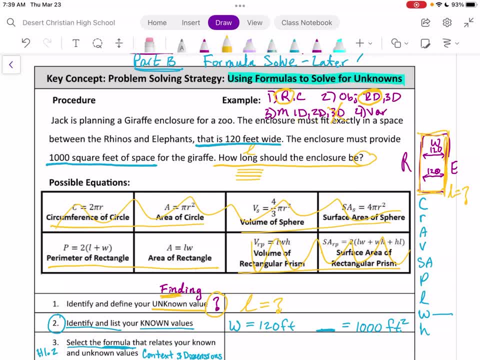 for this, this rectangle. Are we trying to measure the distance around the rectangle Like? are we taking the measurement of the fence around the rectangle, Or are we dealing with a measurement of the space of the rectangle, which would be the area of the rectangle? And this now. 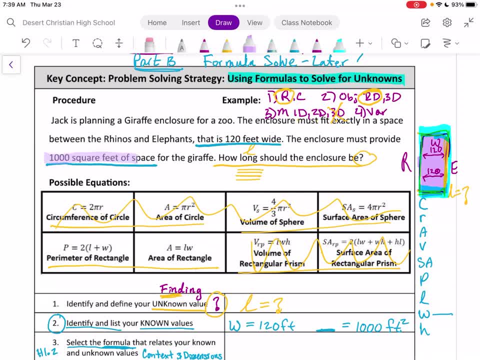 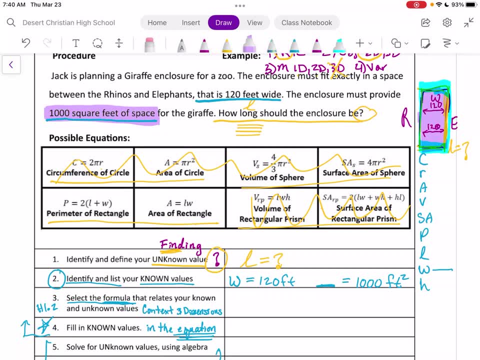 helps us connect with this variable here right, Which is we are dealing with not a distance around, we are dealing with the space of the enclosure. So this helps us connect two pieces here. This, 1,000 feet squared, is the area of the space, the area of the